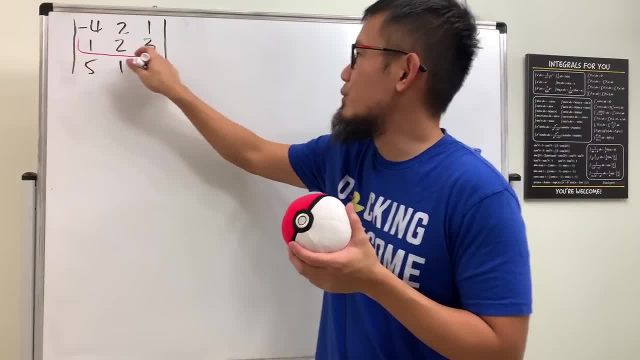 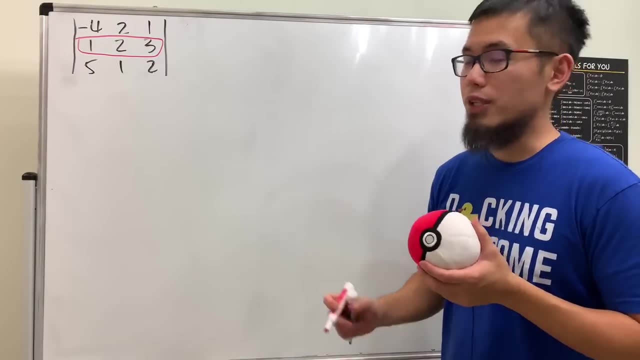 Alright, I'm just going to focus on the second row, just to do it on purpose, just to emphasize: you can do it to whichever row that you want, whichever column that you would like, And you also have to pay attention to the sign, and let me put it down on the side, right here for you guys. 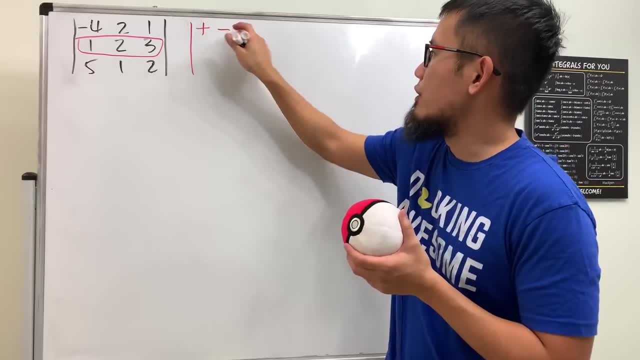 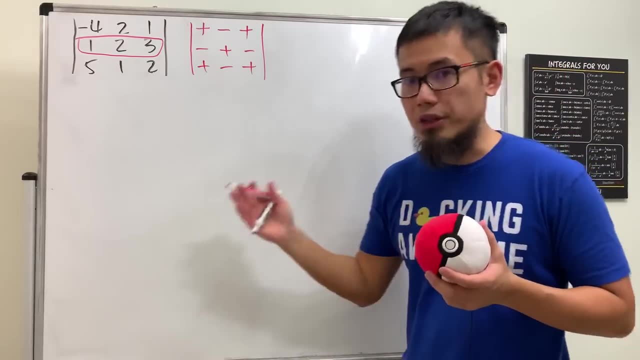 You start with plus right here and then just alternate, And then you have the minus, plus, and then you have the minus, plus, minus, and then plus, minus, plus. So So let's have this done right here, just to get ready. 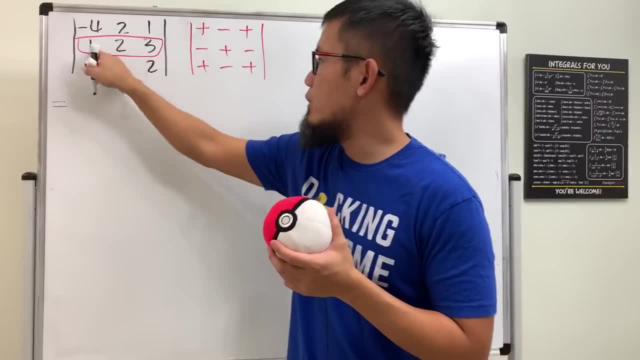 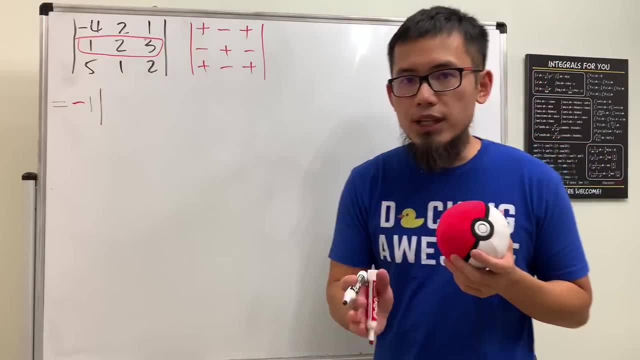 Now this is how it goes: First we are going to put down negative 1 right here, and then we are going to multiply by the determinant of a 2x2 matrix, And to get a 2x2 matrix you just delete this row and you also delete this column. 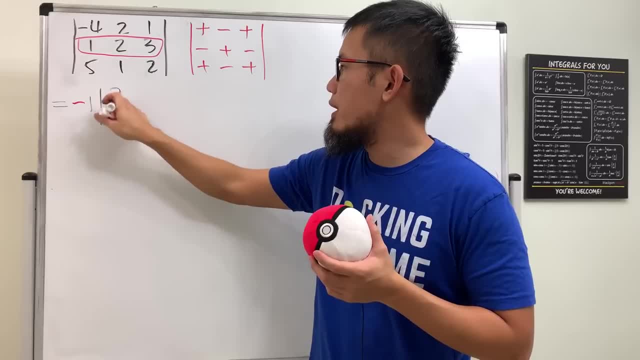 And you have 2, 1, 1, 2.. So you just put it down right here. So, as you can see, we were working with a 3x3 matrix and now this is a 2x3.. 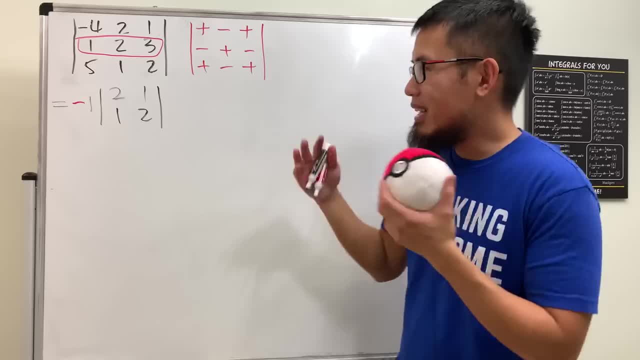 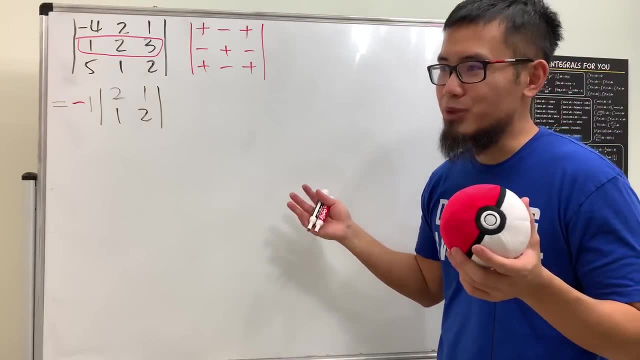 So it's going to get smaller and smaller, And that's why the cofactor expansion works for any bigger size of the matrix as well. But if you are dealing with a 5x5 matrix, you know that's actually pretty hard. 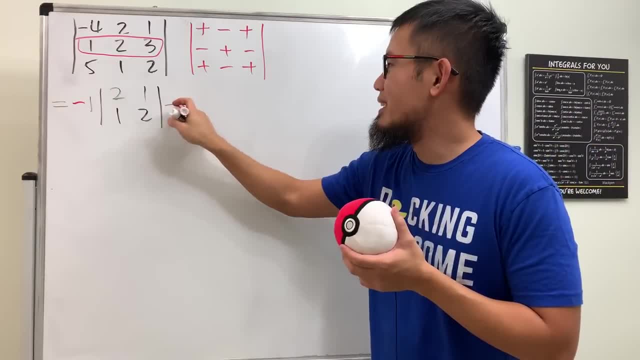 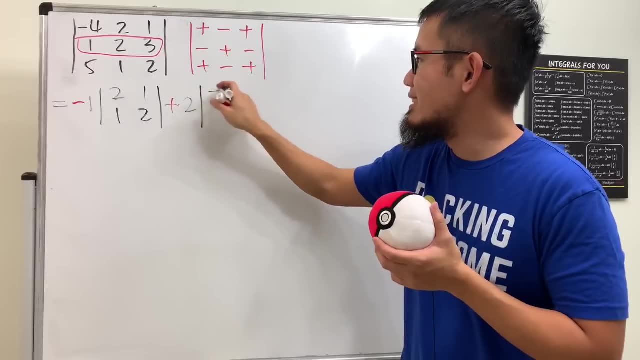 Anyway, next we will have the plus 2 right here and then multiply by the determinant of: well, get rid of this, get rid of that. So we have negative 4, 1, and then 5, 2.. 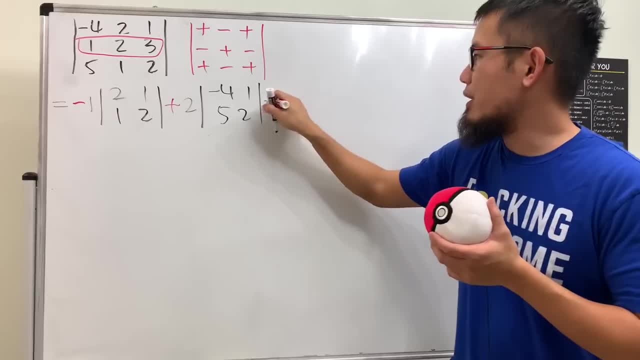 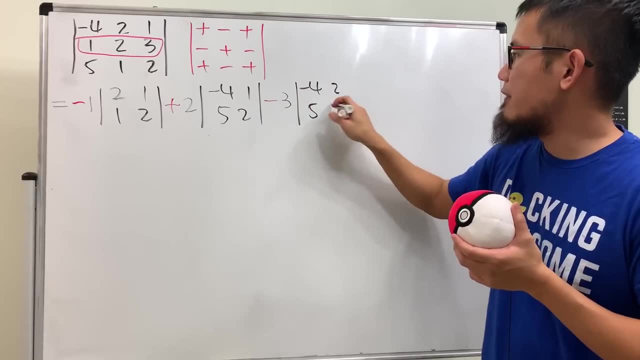 Alright. lastly, minus 3 right here, And then times the determinant of get rid of this and that, So negative 4, 2, and then 5, 1.. Alright, so that's what we have. 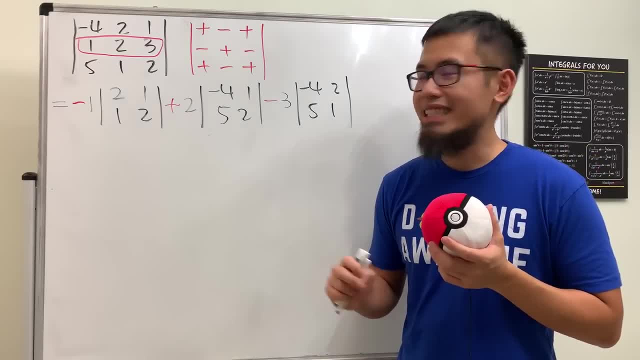 And now, how do we calculate the determinant of a 2x2 matrix? If you want to use the cofactor method, sure, but you don't have to. It's just this times, this minus that times that, That's it. 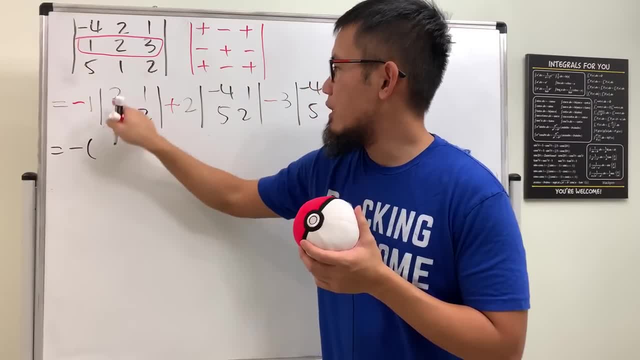 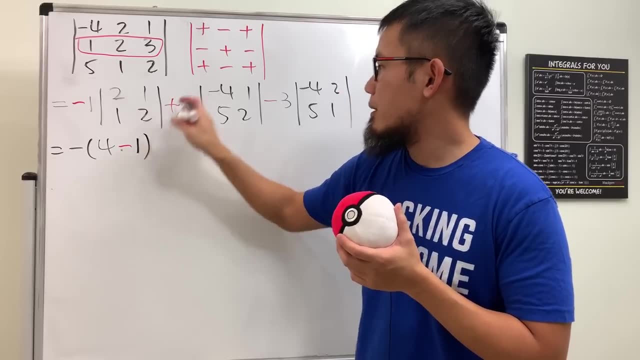 Okay, so for the first one right here, we will have negative 2 times 2 is 4, and then minus 1 times 1.. So 4 minus 1 right here, And then plus 2 times this times this is negative 8, and then minus 1 times 5 is 5.. 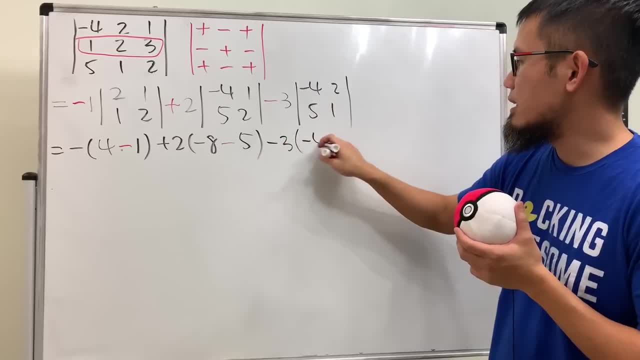 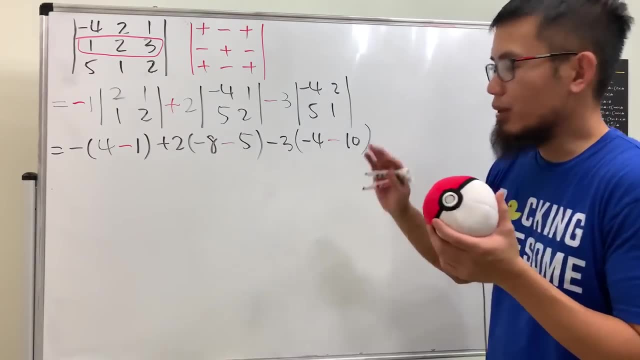 And then for the last one, we have minus 3 times. this times this is negative 4, and then minus 2 times 5 is 10.. Now, just go ahead and just do all the little numbers, Everything. all together, we will end up with positive 13.. 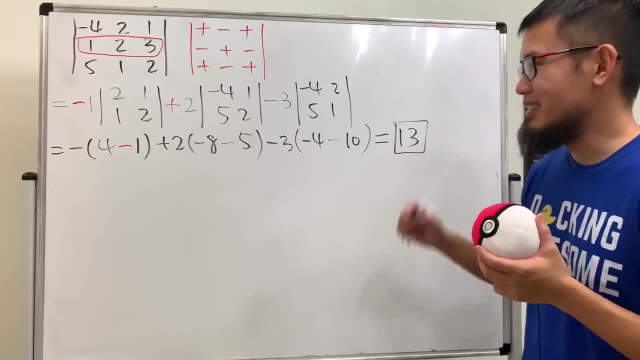 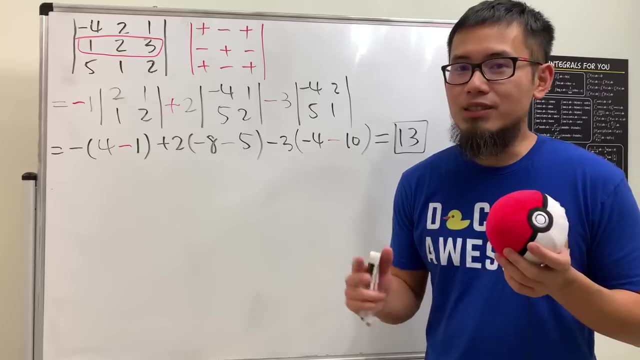 I didn't do this in my head, I did this beforehand. That's how I know. the answer is positive 13,. right, Anyway, that's pretty much it. But now I think many of you guys know there's a trick. 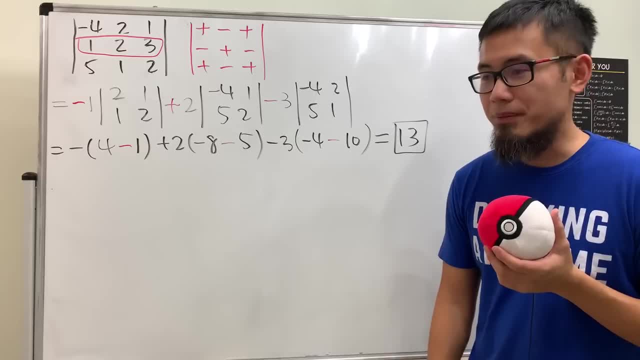 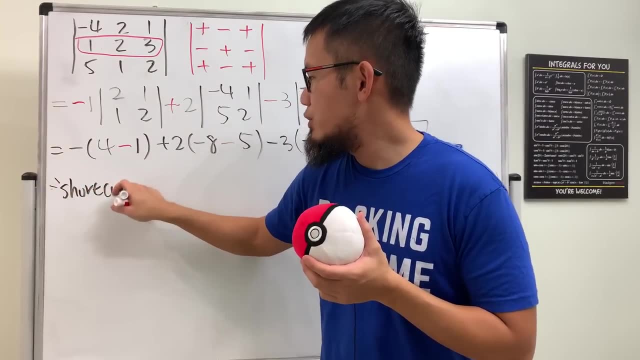 There's the so-called shortcut right of a 3x3 matrix determinant. Let me show you guys that. So this right here is the so-called shortcut. Is it really shortcut? I don't know. You can tell me that later. 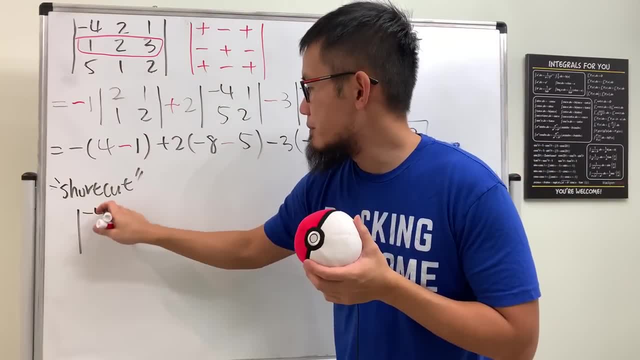 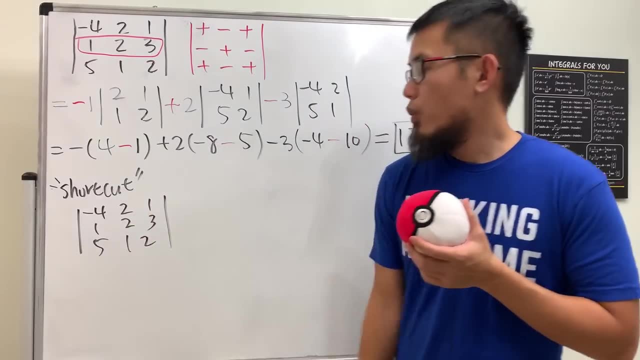 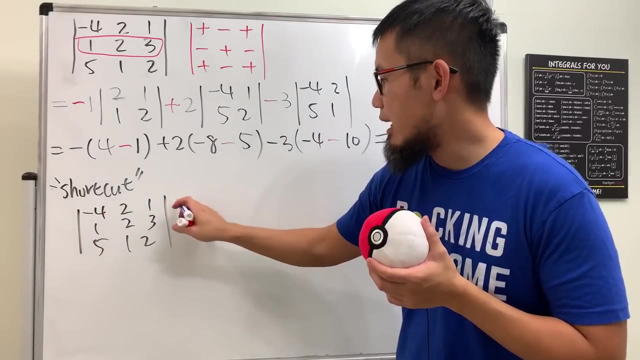 Anyway, how it goes is that you just write down the matrix, right? And then: Well, right, here, we actually going to copy down the first two columns again and then put it down on the side. So this is negative: 4, 2, and then 1, 2, and then 5, 1, right. 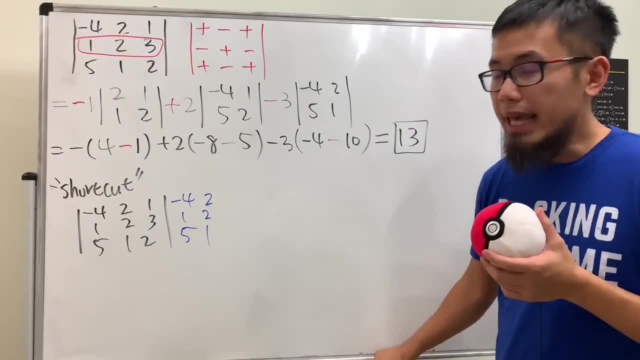 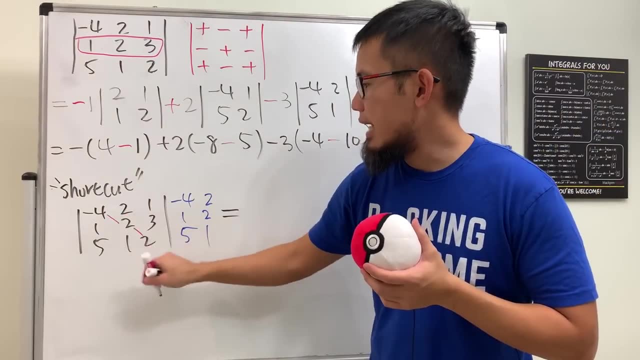 So just the first two columns from here and there. And this is how it goes. First, we are going to multiply this, this and that right. So negative 4 times 2 times 2.. We get negative 16.. 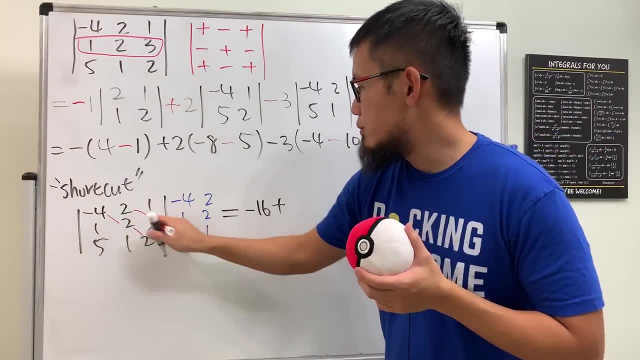 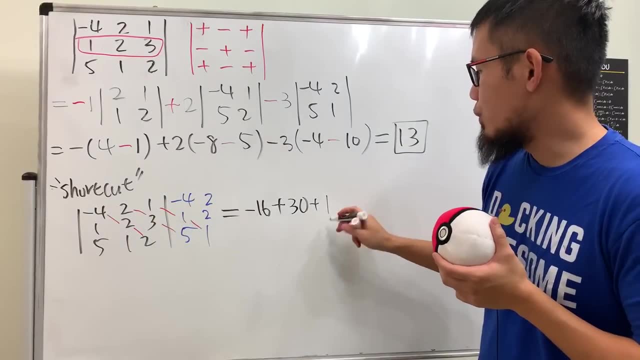 And then we are going to are going to add it with 2 times 3 times 5, which is 30, and then we are going to add it with 1 times 1 times 1, which is just 1, like this, and then we are going to subtract and then we go the other way. 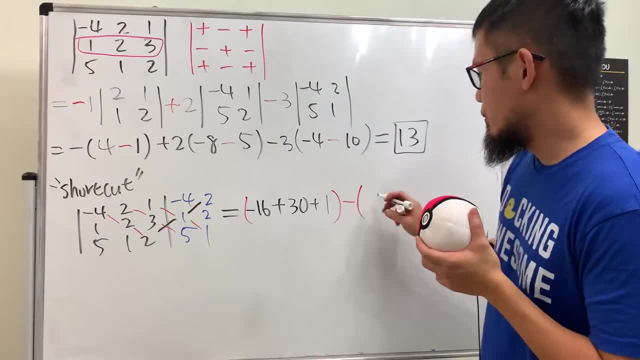 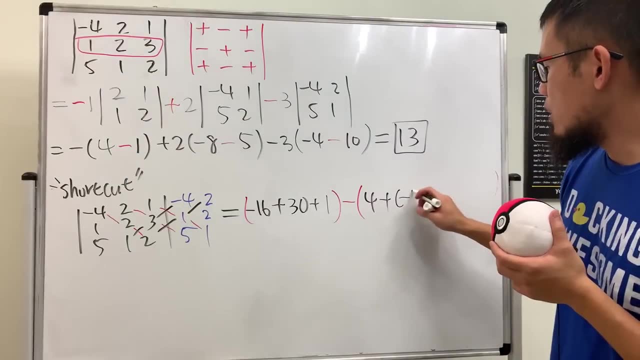 so have a look: 2 times 1 times 1, which is 4, and then you combine with negative 4 times 3 times 1, which is negative 12, and then, lastly, we have 1 times 2 times 5, which is 10, so it seems pretty. 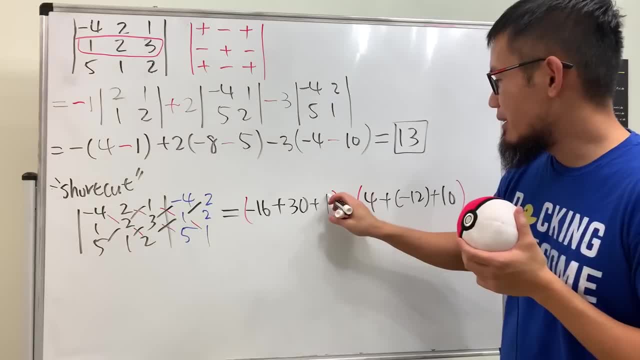 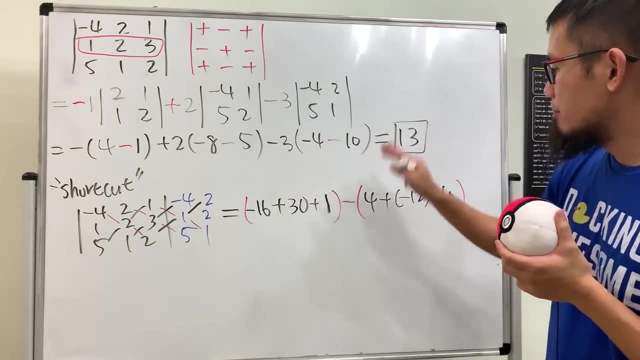 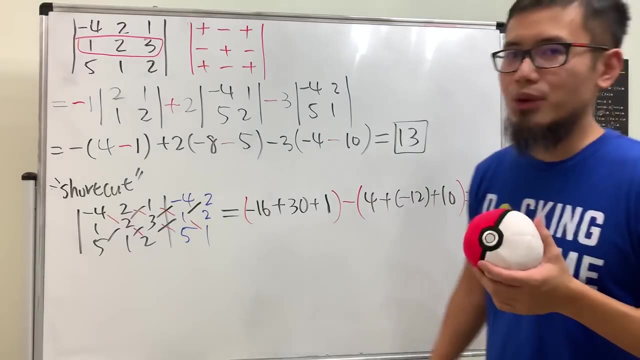 magical right, and you can see, this right here is going to be positive 15 and this right here is going to be positive 2. 15 minus 2, indeed, we get positive 13. is this just a nice coincidence? well, i will show you guys the quick proof of. 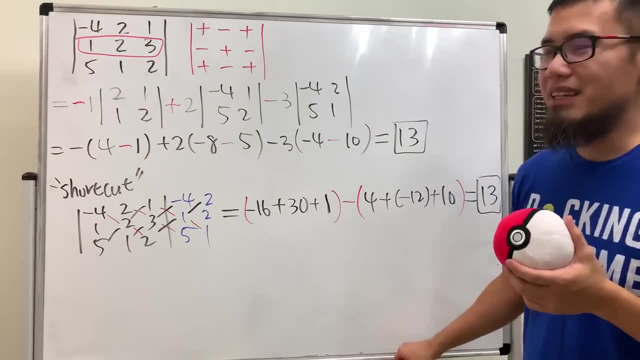 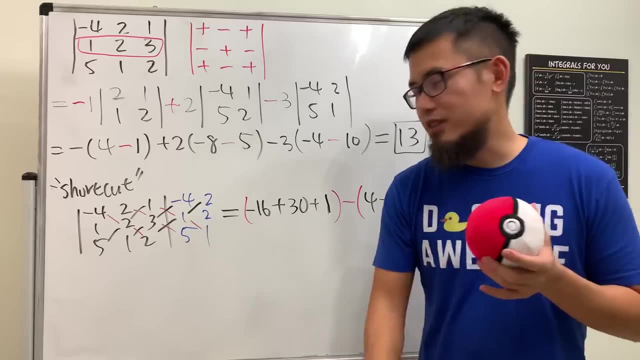 this right here. it's very computational and after you guys see the following, you guys will see that: ah yeah, it's just a nice way to organize all these computations. but let me emphasize though: this only works for this 3x3 matrix. when you have a 4x4 matrix, you will have to just go through the. 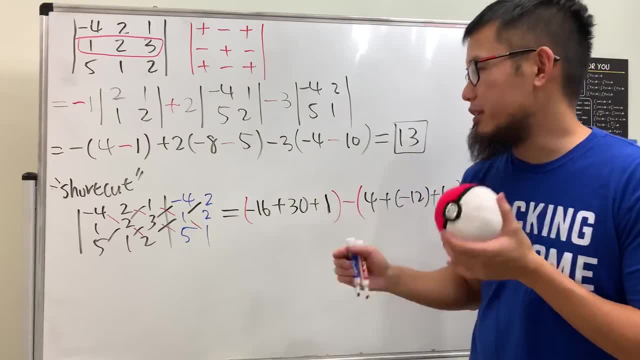 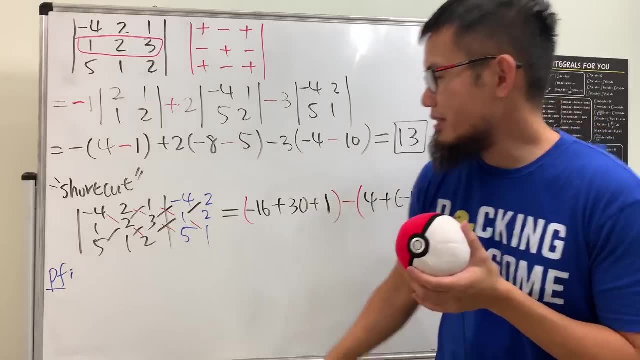 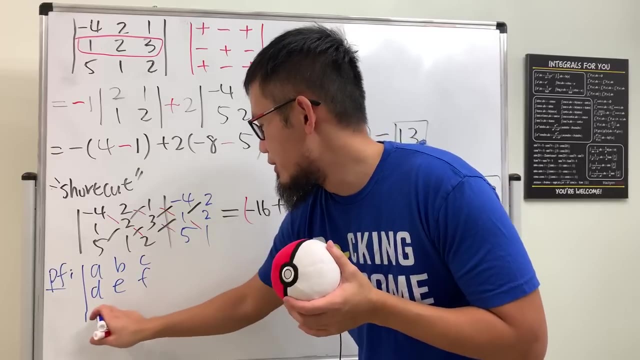 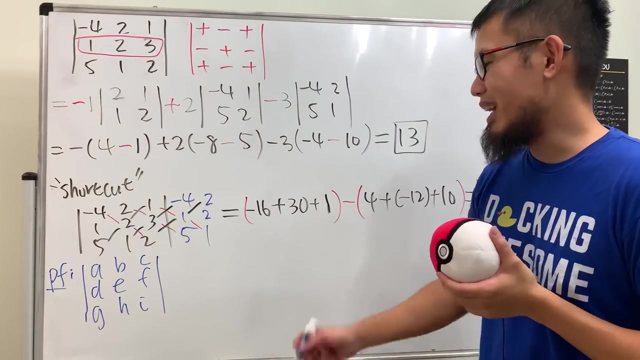 cofactor expansion, where you can do the third way, but that will be later on. so let me just show you guys the quick proof, real quick, and to do the proof for this, i'm just going to consider the matrix a, b, c, d, e, f, g, h, i, y, because you will have to use letters when you do do proofs. so yeah, anyway, 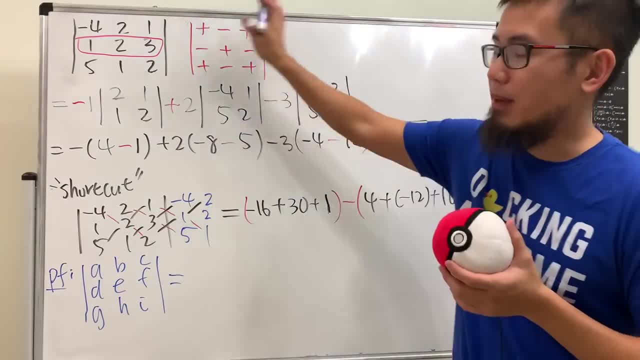 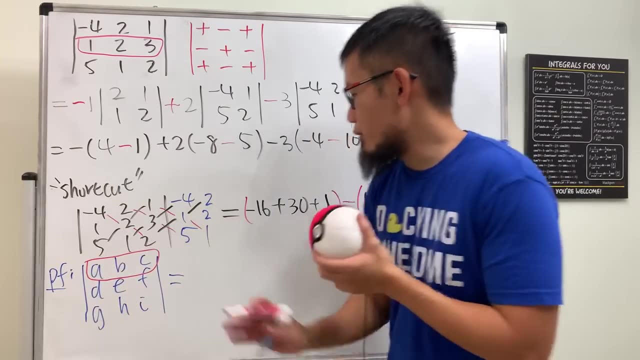 what we'll do is we're actually going to use the cofactor expansion to help us out. so first i'm just going to do this across the first row. i'm not going to be too creative this time. we have positive a, so we have the a right here, and then multiply by the. 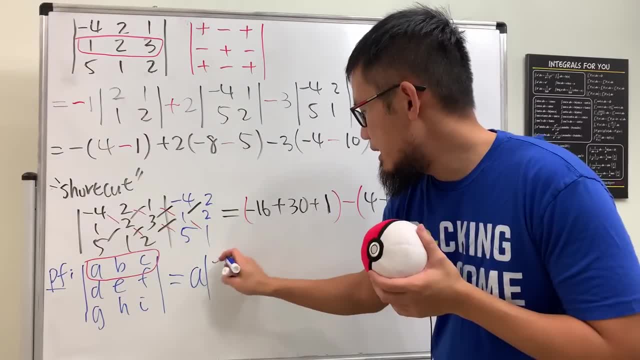 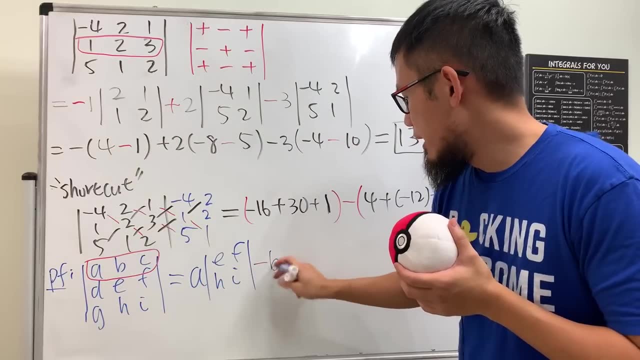 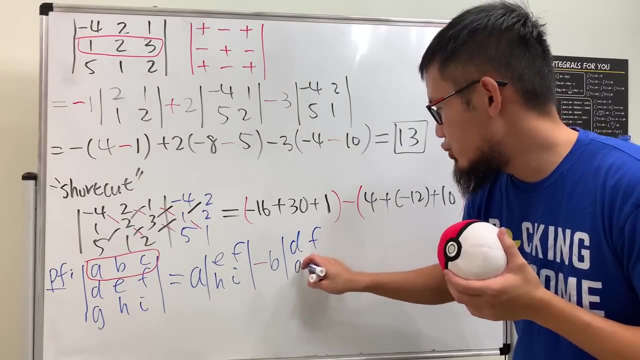 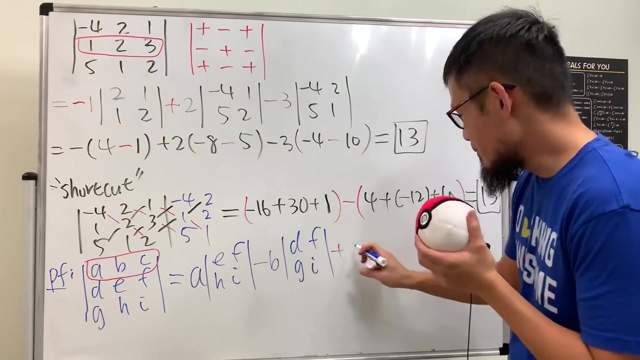 determinant of just this part, right. so we have e, f, and then h, i, and then next minus b, and then times, the determinant of d, d, this, d, d, that, so d, f, g i, so d, f and g, i. and then, lastly, we have the plus c. well, we're not doing integration, so don't don't get too excited. plus c, and then 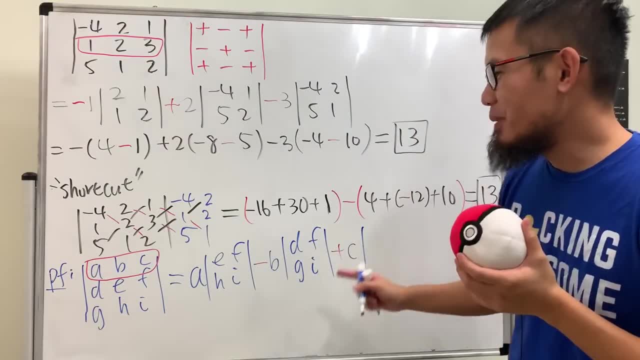 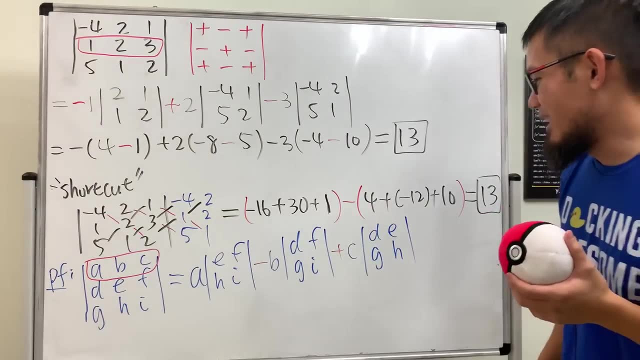 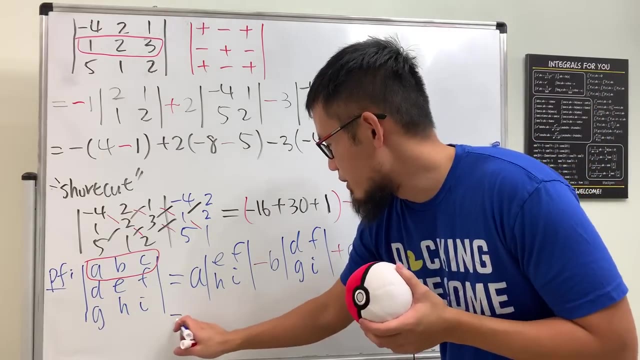 times the derivative- oh, not the derivative times the determinant of e, f and then plus c, and then the determinant of d e g h, d e g h. it seems that i'm the one who's getting excited, but anyway. and then what do we do next? you just multiply the others. i said it's very computational if 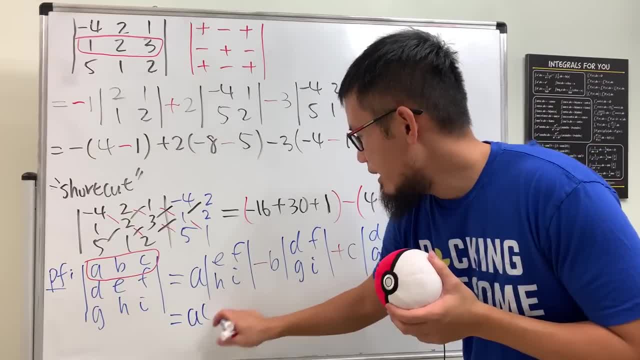 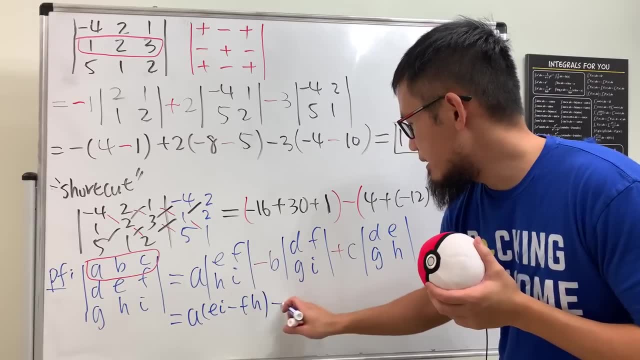 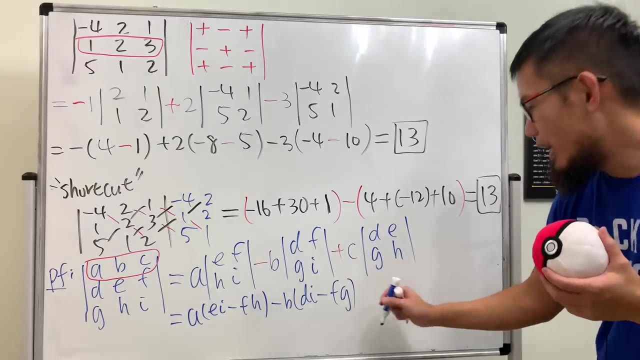 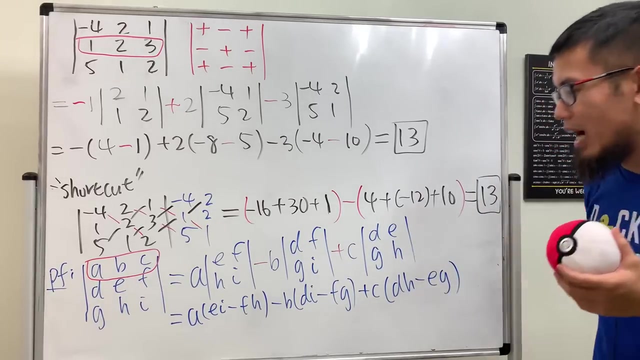 you just want to do it this way. well, we have a, and then we do this times this, minus this times that, right, so it's e i minus f, h, and then minus b, times d i- another d i method- and then minus g, and here we have plus c again, and then d, h, and then minus e, g. alright, so that's what we have. and 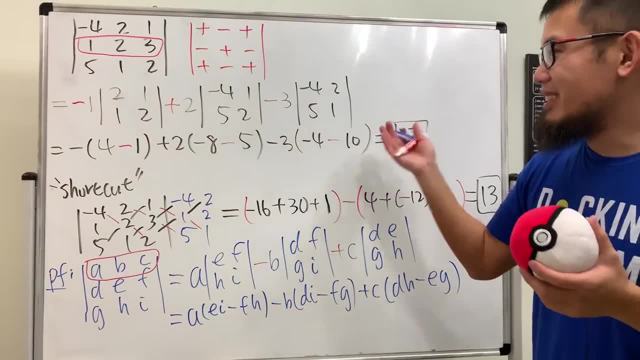 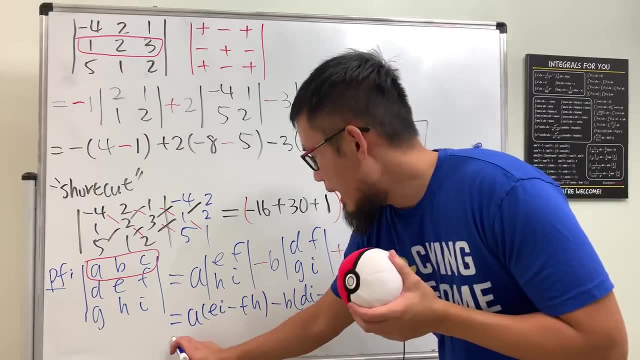 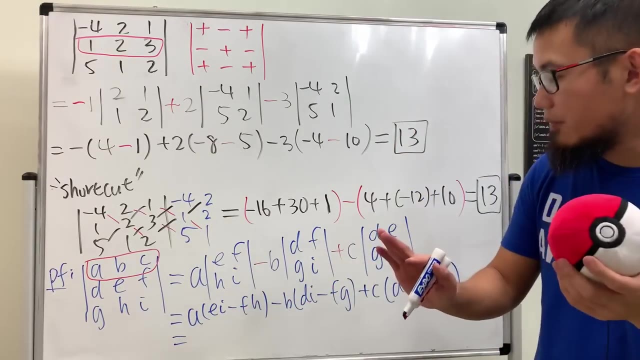 this is pretty much the formula to find the determinant of a three by three matrix, but nobody even memorized this right. anyway, though, have a look, i'm actually going to combine the terms that are positive. well, without the negative. let's put that down first, and then subtract the. 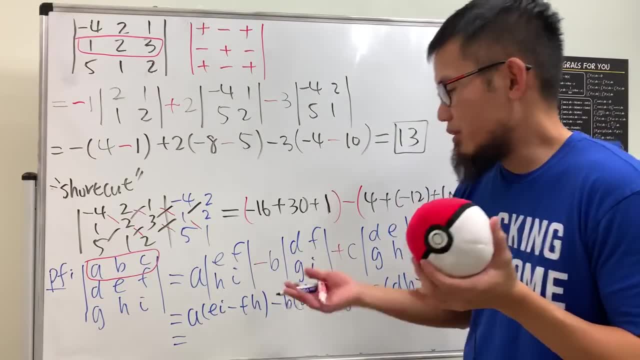 This right here is the positive term, but I don't know what A, E and I are, so technically I don't know if it's positive or not. But anyway, this right here: A, E, I. and then I'm going to add it with: 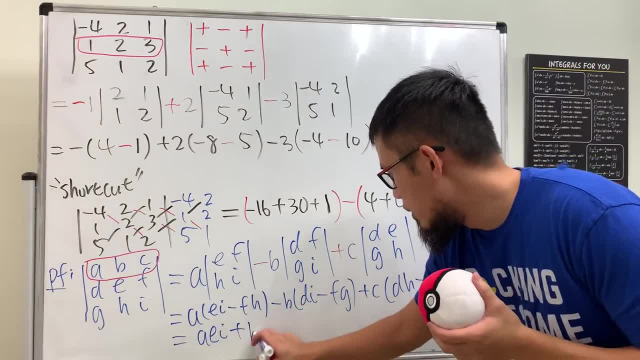 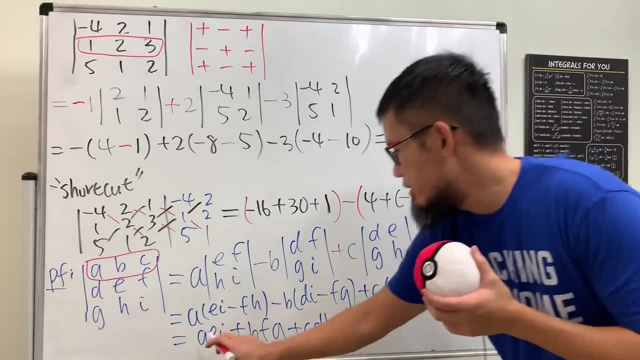 this is going to give me plus, so it's B F, G and lastly C D H. So plus C D H, As you can see. here is the first part And then next. I'm just going to subtract. 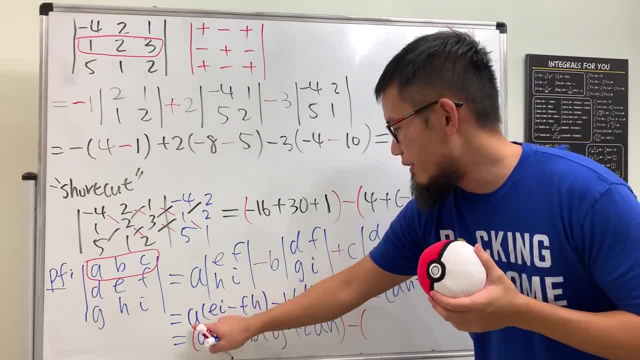 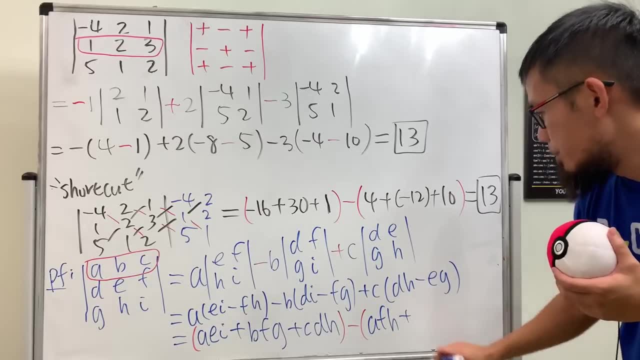 Well, let's see, This has the minus, so we have this and that, So it's A, F, H, and then the minus is outside already, And then here will be plus. We have this, so B D, I. 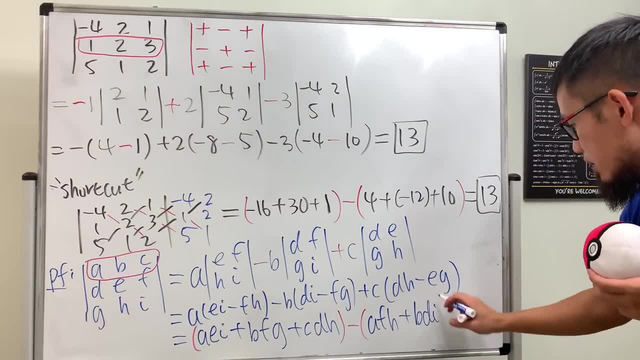 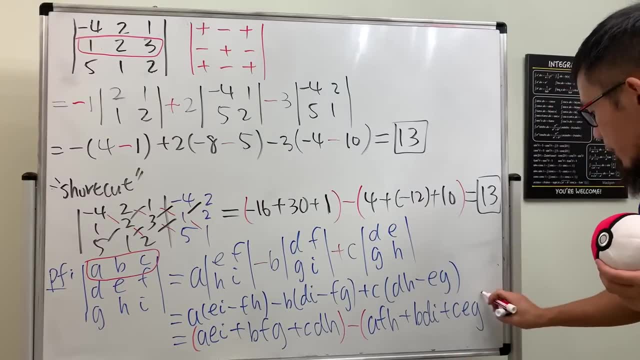 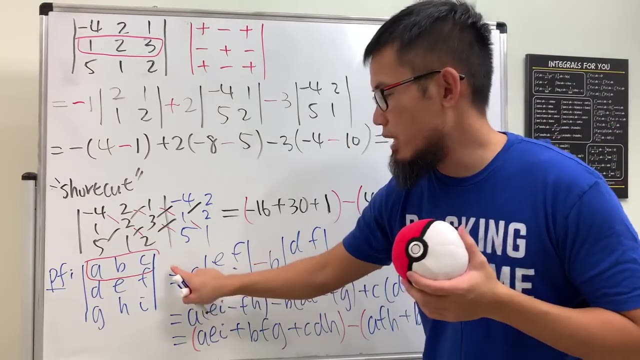 And then, lastly, we have C, E, G. All right, so that's what we have. Very, very cool, huh? Now have a look, If we come back to this matrix and then if we just put down the first two columns again on the side, 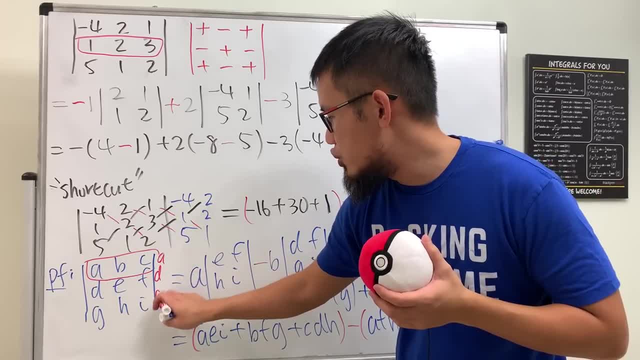 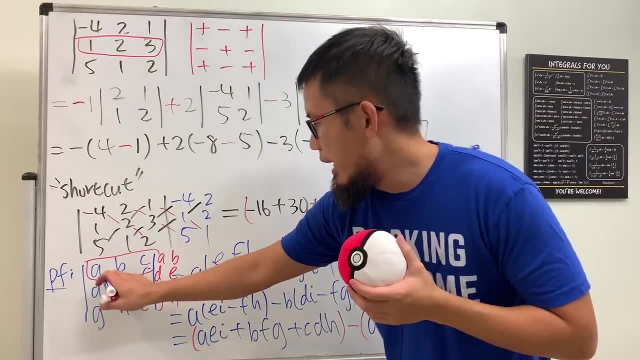 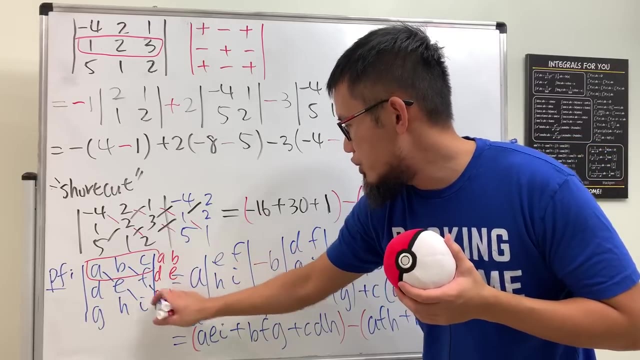 namely A, D, G and then B E, H. Have a look, When we do A times, E times, I isn't it right here? And then next B, F, G, Aha, And then C, D, H. 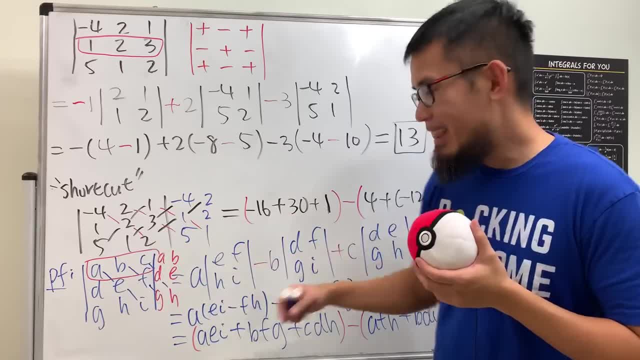 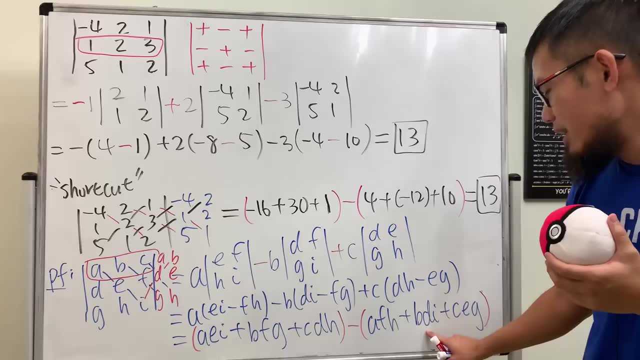 Right here, right. So that's exactly what we did. And then we just go the other way. So B, D, I is right here, right, Even though the order- but the order doesn't matter. And then next we have A, F, H. 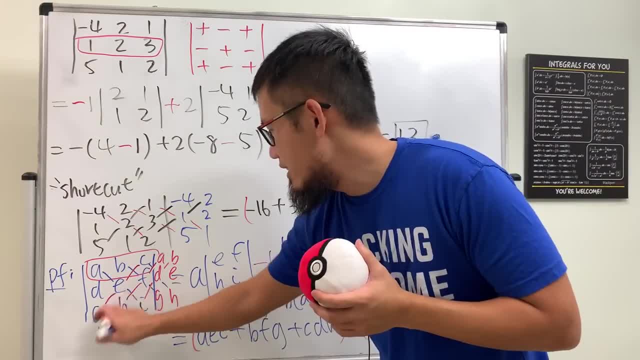 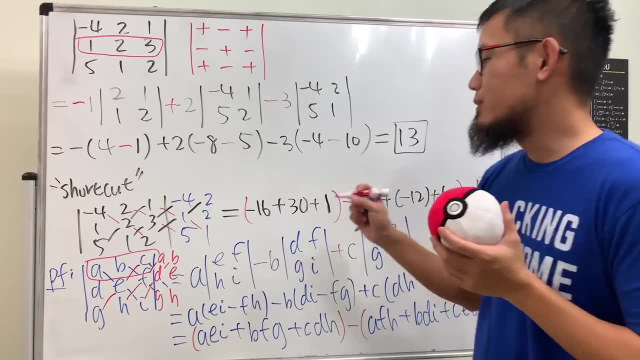 A, F, H, right, And lastly C, E, G. That's pretty much it right. So this right here is a very convenient way for us to find the derivative of the 3x3 matrix real fast. 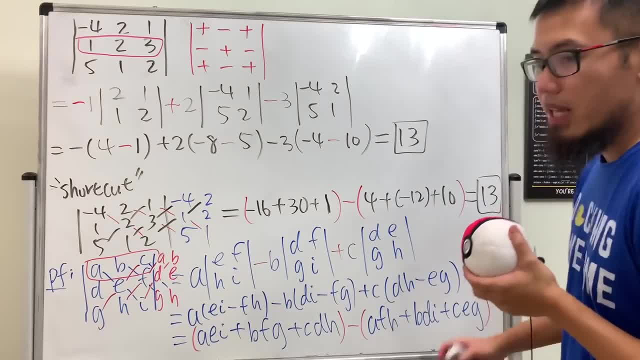 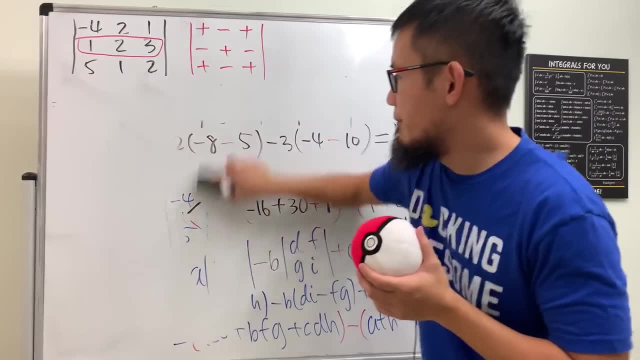 All right, So that's pretty much. That's pretty much it for the first two ways. And now the third way is the most exciting part, Namely, we are going to use properties of the determinant, and then we'll see how they are going to help us out. 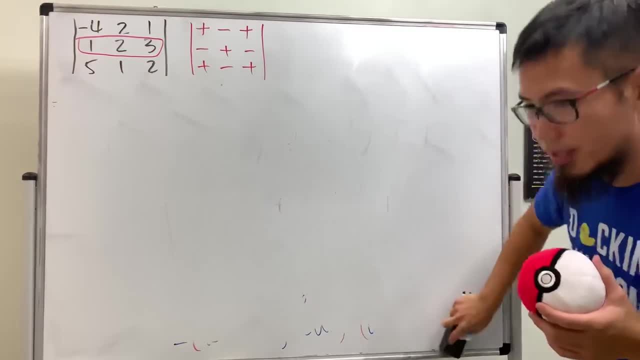 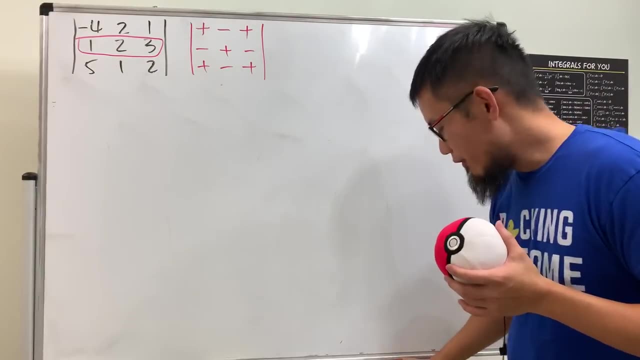 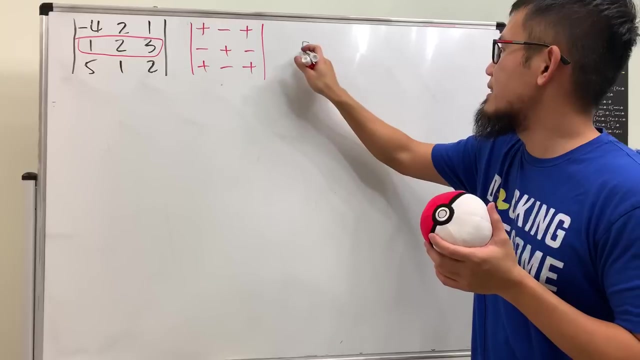 So let me raise the board right now and let me know how you guys are doing. All right, So I'm going to write down one of the very useful facts to calculate a determinant. So here is the fact right here. Well, this matrix is hard to find a determinant. 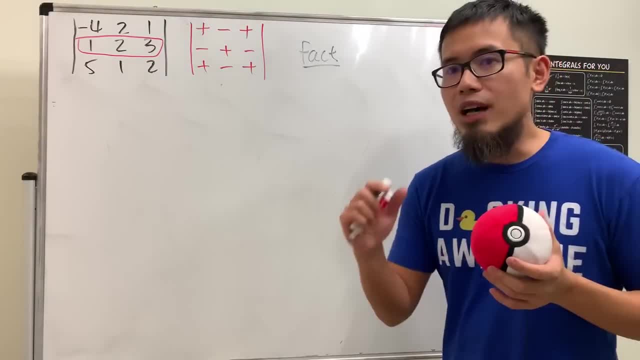 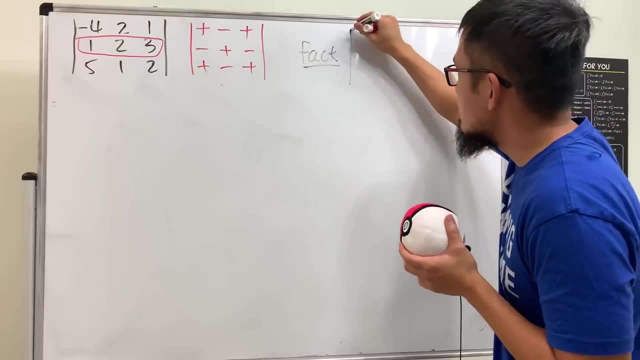 There's one kind of matrix, very easy to find a determinant, namely a triangular matrix. So what's a triangular matrix? Well, it looks like this, And let me just put down a 3x3 example for you guys. Well, let's say, on the diagonal we have the entries A, B and C. 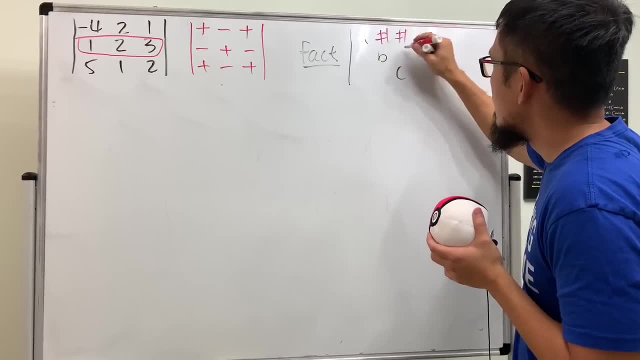 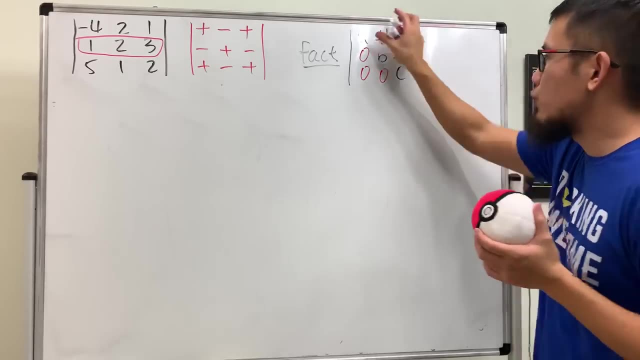 And let's say, here we have numbers, All right, And then the rest, This right here, they are just zeros And this is called the upper triangular matrix. And if you want to find the determinant of this, it's just going to be A times B times C. 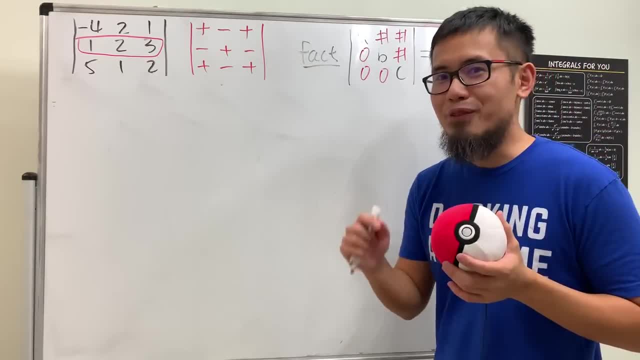 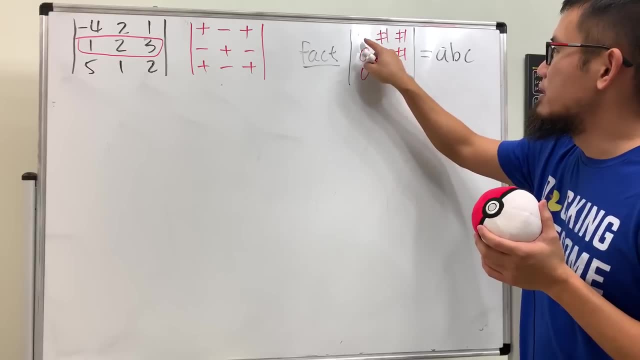 Well, how do we know? Yes, we also have to use the cofactor expansion, But this time we are going to do it across the first column And because we have a bunch of zeros right here, it's just going to be A times the determinant of this. 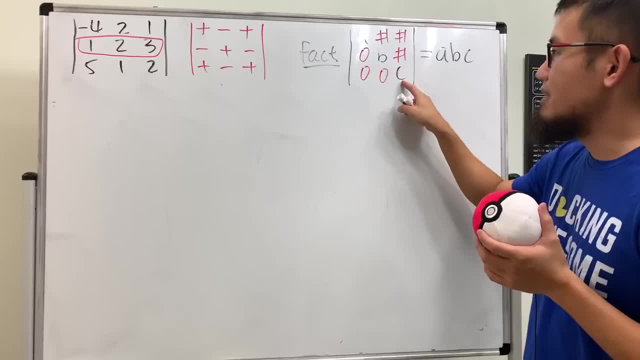 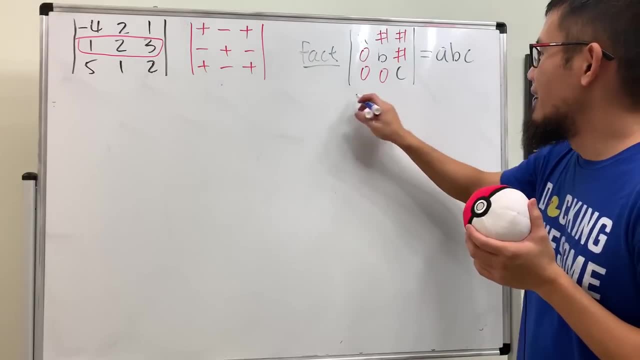 And the determinant of this- because we have the zero here- is just B times C, So namely A times C And B times C, Just like that. Similarly, if we happen to have a lower triangular matrix, So A, B, C on the diagonal. 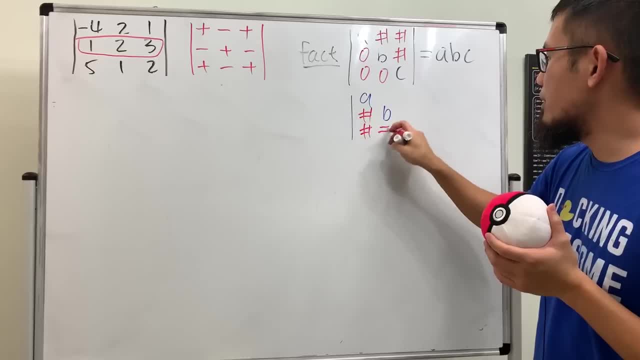 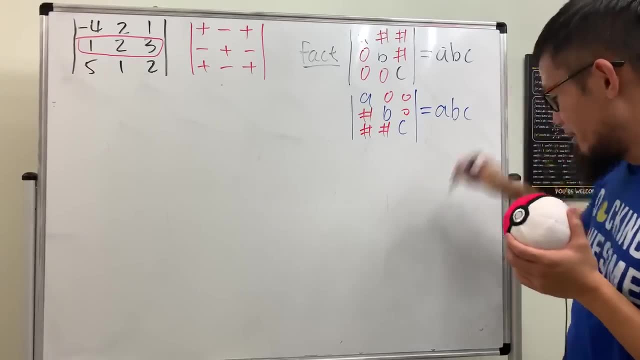 And this time we have a bunch of numbers right here, right here and right here, And then the rest are just zeros. This right here will also give us A, B, C for the determinant. Very nice, So that's our goal. 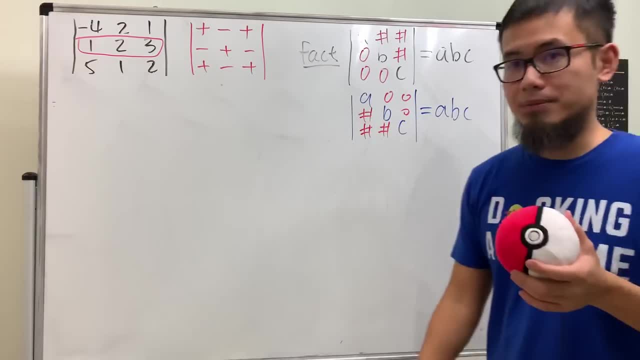 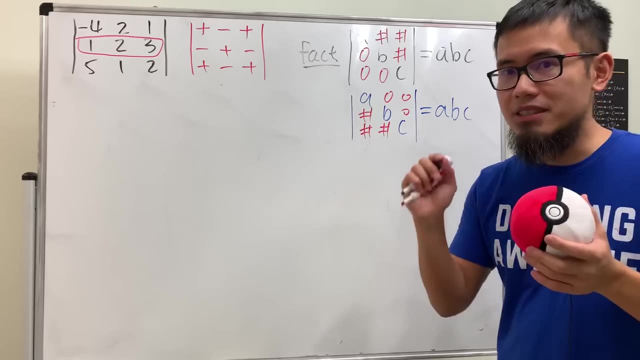 And perhaps let's turn this into an upper triangular matrix, And we also have to be careful of the rule operations that we do. Maybe some of them will affect the determinant. All right, so let me just talk to you guys along the way. 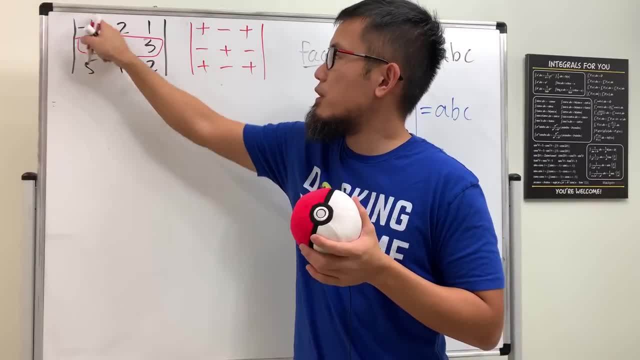 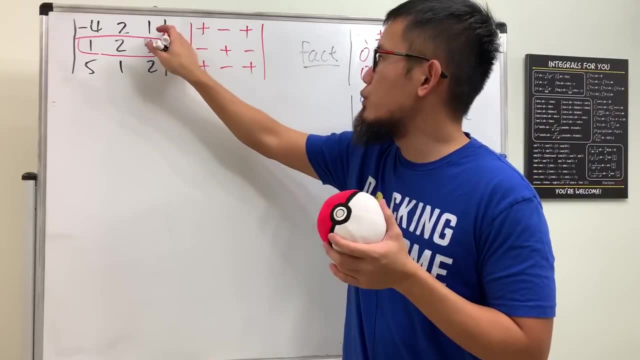 Firstly, I would like to have a 1 in the first entry, right here. That's going to help us out, because I want to get rid of this 2 to be 0, right, So I'm actually going to interchange the first two rows. 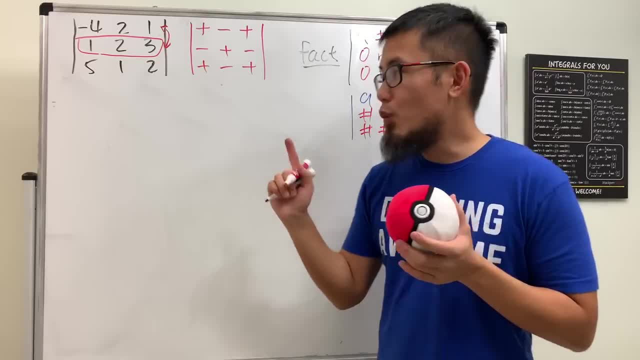 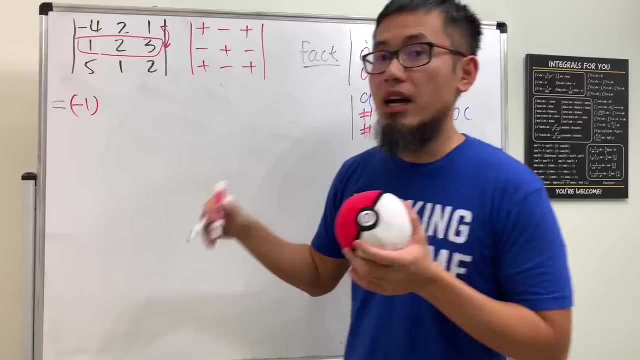 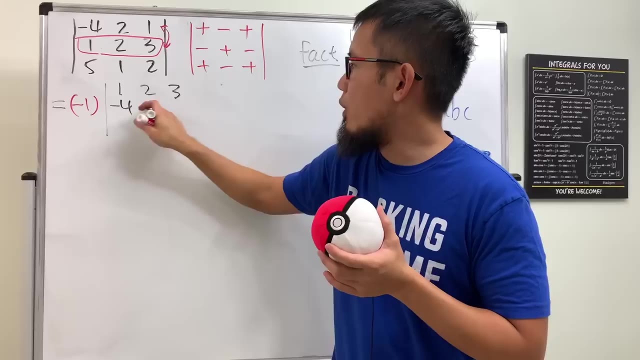 And when we interchange rows, well, we will have to just multiply the determinant by negative 1.. So this right here it's going to be negative 1 times the determinant of this matrix. You put down 1,, 2,, 3 first, and then negative 4 to 1, and the last row stays the same. 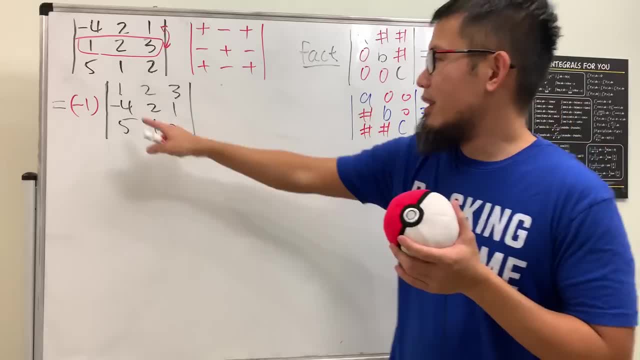 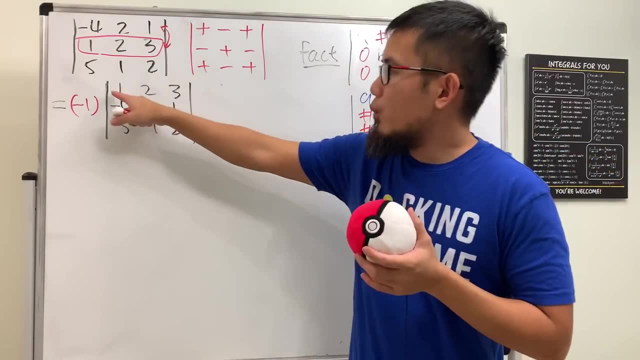 So that's what we have Now. let me get this to be 0, and likewise, we'll get this to be 0. And the best part of doing so is that, well, we'll just do some rule operations, Namely, we'll multiply this by. 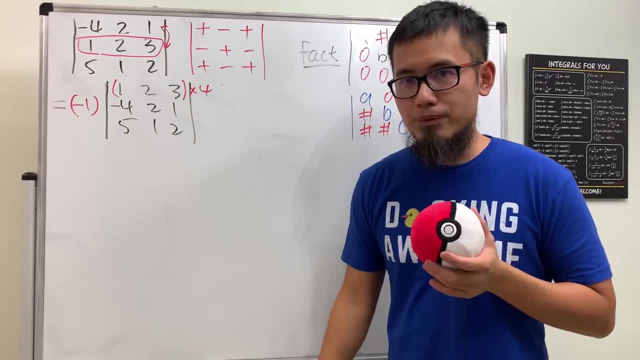 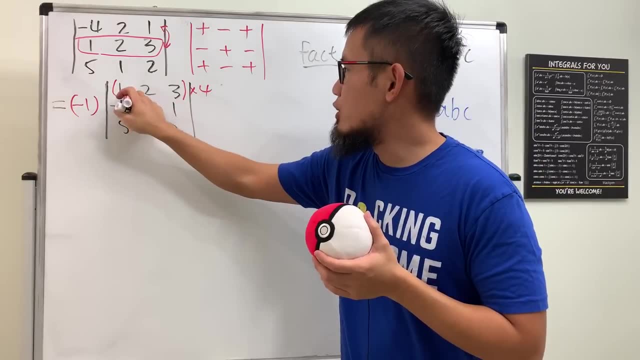 positive 4, and then add it to the second row And the determinant actually stays the same. So that's the best part. So let's go ahead and just do that. So this is going to be 4,, 8, and 12.. 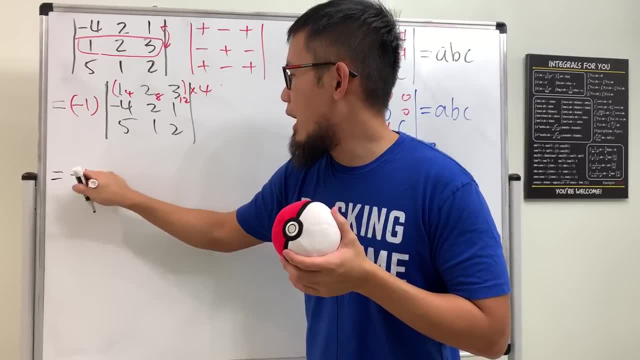 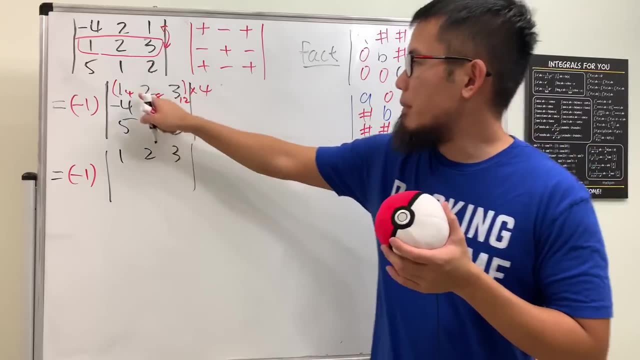 And add it here. So here we will have negative 1 times the determinant of this matrix. We have 1,, 2,, 3 stays the same, But this is going to be 0,, this is going to be 10, and this is going to be 13.. 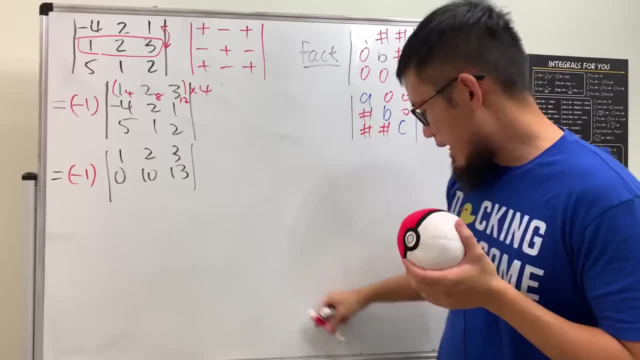 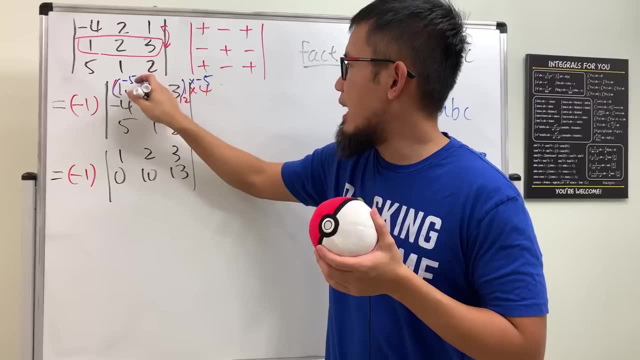 Now let's also make this equal to 0.. This time, though, we will multiply the first row by negative 5.. So we're looking at this as negative 5,, negative 10, and negative 15.. And then we're going to just combine. 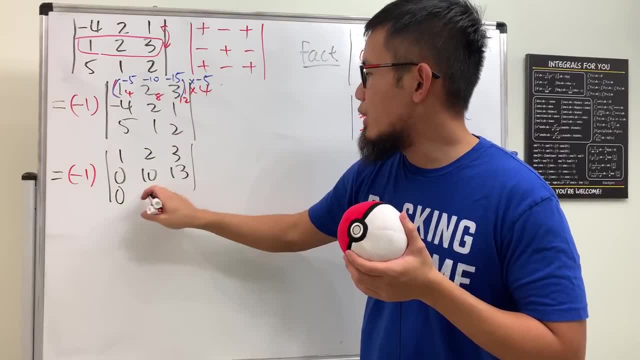 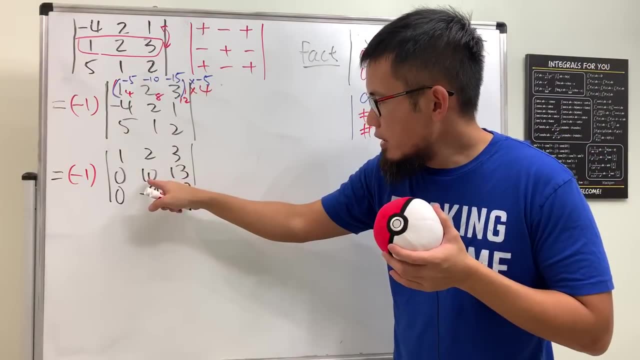 This and that: together, we get 0.. This and that, together, we get negative 9.. This and that, together, we get negative 13.. All right, very good. Now this right here is 10.. We're going to get the REF. 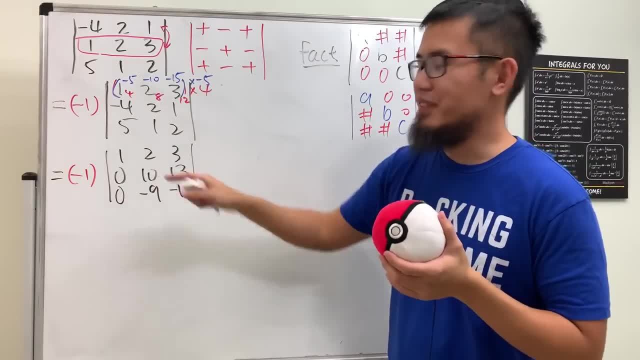 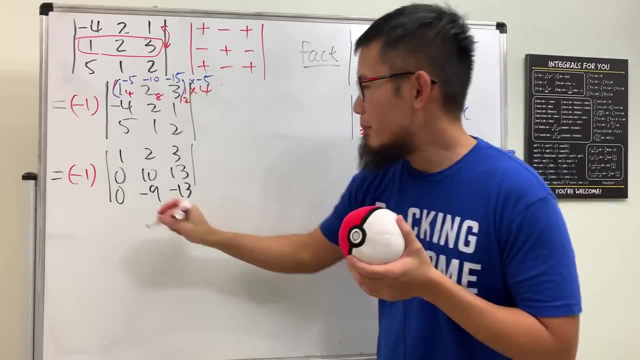 So you do not need to like divide it by 10 whatsoever, You can just leave it like that. But I do want to make this equal to 0 so I can get into the upper triangular form, right. So I'm actually going to multiply this row by positive 9 over 10.. 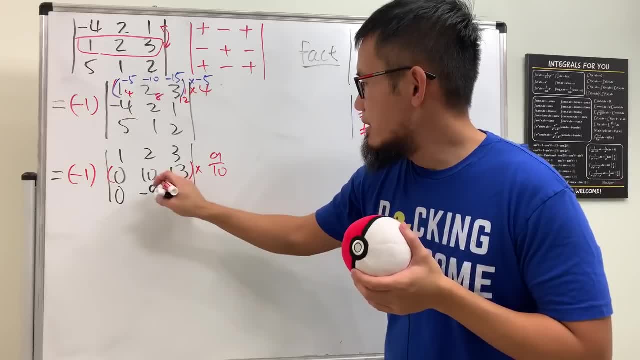 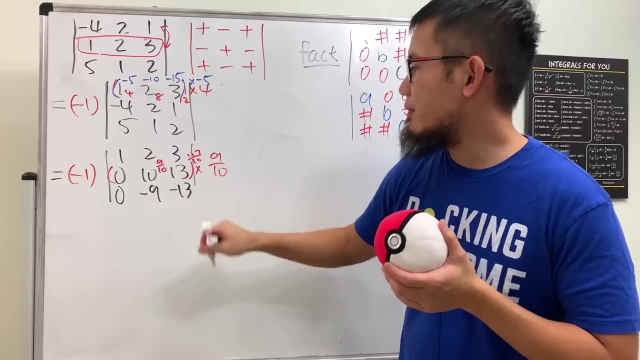 And then add it to this row. Have a look, This is going to give us positive 9 over 10.. And 9 times 13 should be 117 and then over 10.. All right, So here this is still negative 1..